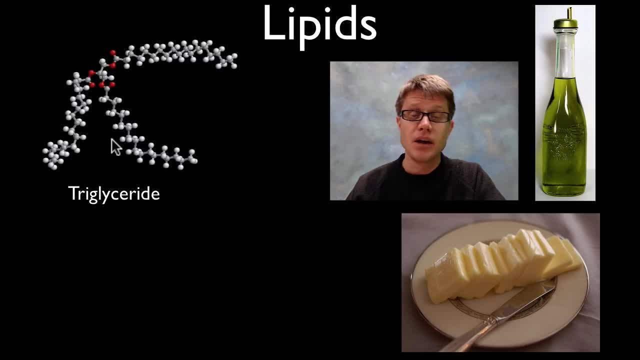 to have three fatty acid tails And that's where the energy is, And so when we eat fat, we can break it down. We have enzymes called lipases that are able to break that down and then we can get energy from it, And that's been very important. We can store energy and 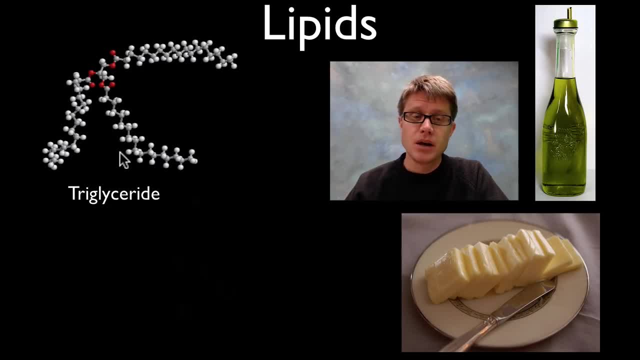 fats inside our body, and then we can burn them when we need them. But don't forget that fats, in addition to providing energy, also provide the surroundings, And so the cell membrane that goes around every cell is made up of phospholipids And the cholesterol is. 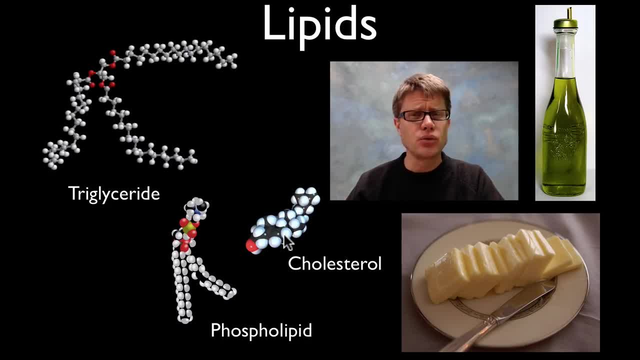 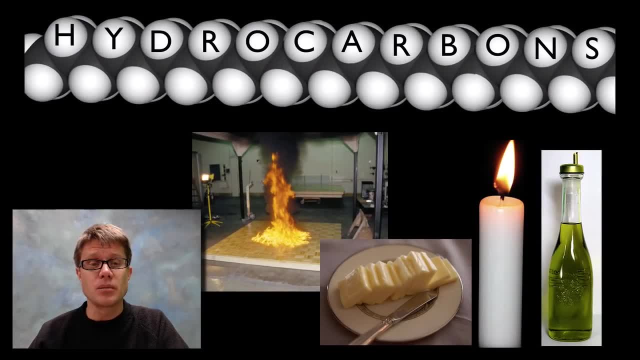 found within the phospholipid bilayer, and that maintains the fluidity of the cell, And so lipids are incredibly important. But where does the energy come from? That comes from the hydrocarbons, And so if you look at those fatty acid tails, it's essentially a carbon attached to a carbon. 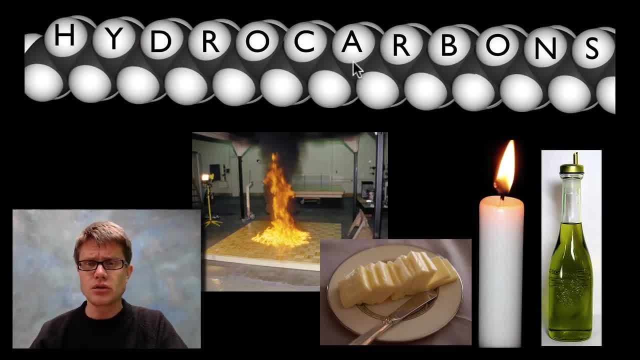 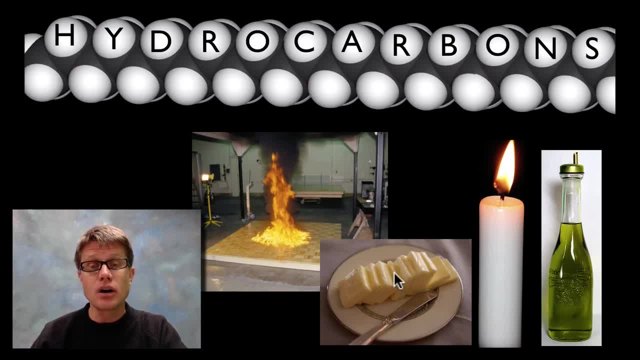 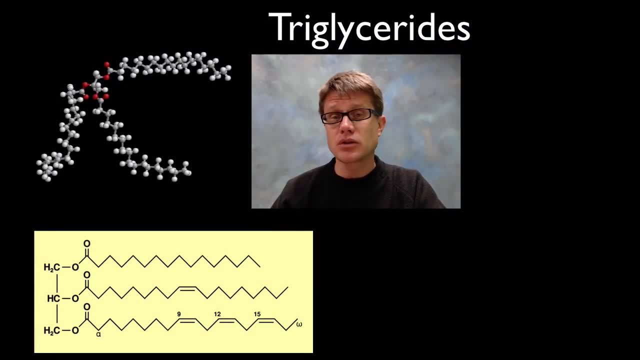 a lot of energy between those carbon hydrogen bonds, And so there's also a lot of energy found in butter or in olive oil. It's in the bonds between the carbon and the hydrogen, And so let's start with the triglycerides. So this is a basic fat. The head up here is: 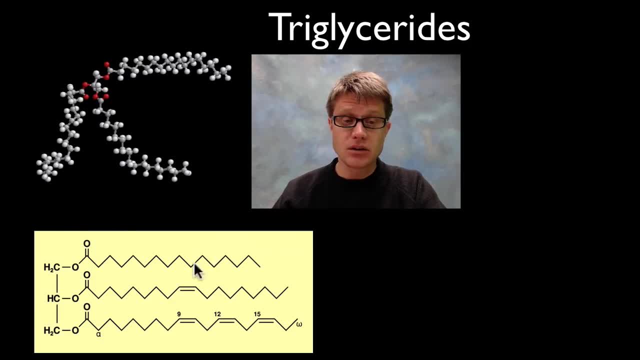 going to be called the glycerol head, And then this is going to be the fatty acid tails that go down the end. And so a fatty acid tail has so much carbon and hydrogen in it that on this diagram we don't even draw them. Each of these points represents a carbon. 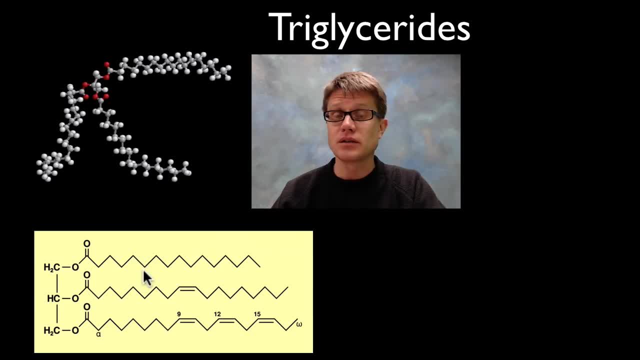 a carbon, a carbon, And then right here we're going to have two hydrogen bonds, or two hydrogens bonded to each of those carbon, And so you can see that there's a huge amount of energy locked within that triglyceride And we can get that out through cellular respiration. 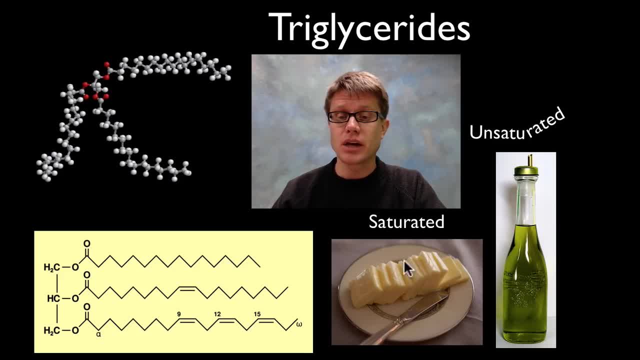 But know this, Those tails can come in two different forms. We can have what are called saturated tails. A saturated tail is going to have hydrogen all the way around the outside, And if you have hydrogen all the way around the outside, then you're going to be saturated. 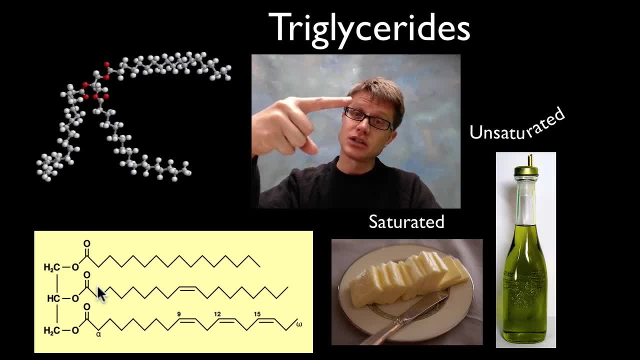 with hydrogen, And if you're a saturated fat you're going to be a straight fat, And so a triglyceride is going to have three of these fatty acid tails and the glycerol head. But if it is saturated all of those are going to be straight, And if they're all 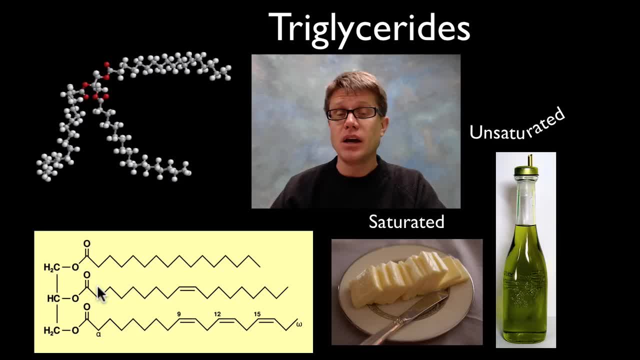 straight. they can pack up on top of other triglycerides And so saturated fats are normally going to be a solid at room temperature. What happens if you don't have hydrogen all the way around the outside? You're going to form these double bonds in here. If you have double 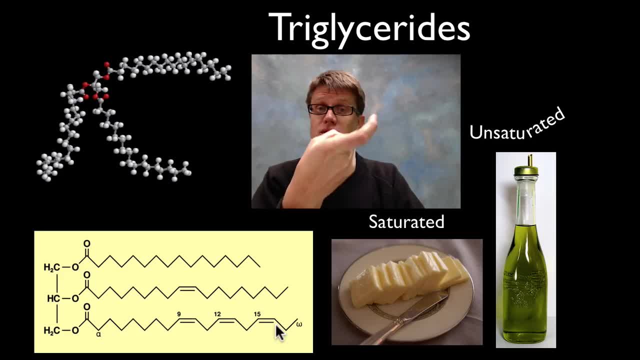 bonds. basically, what that does is puts a bend in your tail, And so you're going to have a kinky tail. And so if you're a saturated fat, you're going to look like this. If you're an unsaturated fat, you're going to look like this, with kinky tails, And the kinky tails. 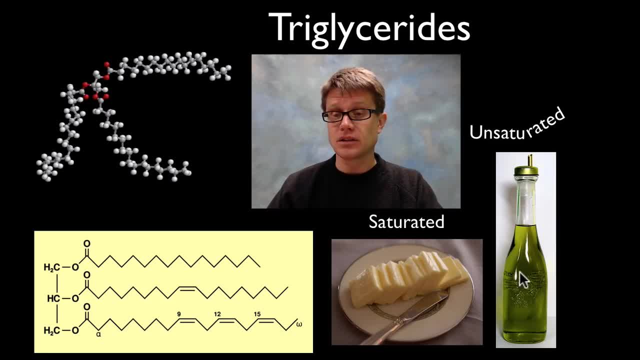 can't quite pack together, And so normally, fats that are unsaturated are going to be a liquid at room temperature. Now, humans have figured out how to take, for example, vegetable oil, which is an unsaturated fat, or it's going to be a liquid at room temperature. 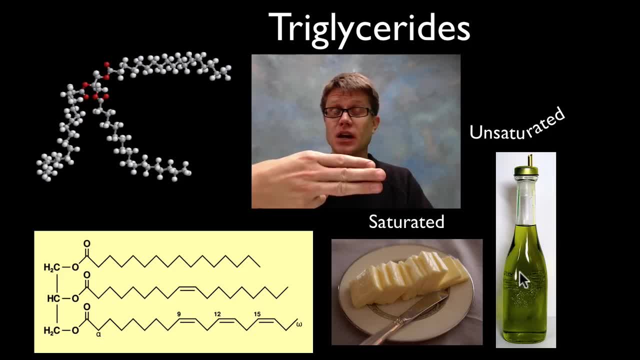 And we can bubble hydrogen through it, We can straighten out those tails And we can make a saturated fat called margarine. that's going to be a solid. at room temperature. We've transformed this fat and if you know anything about fats, those saturated fats are the ones. 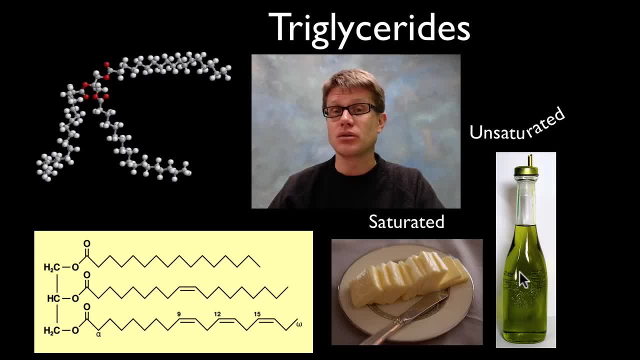 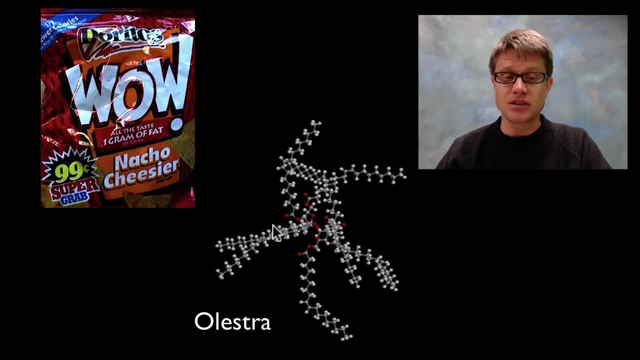 that are least best for us and can lead to arteriosclerosis, especially trans fats. Example, then, of how we've tried to get around this- and this is a somewhat funny story- this is Alestra. Alestra is a fat that was made by humans, And so, basically, what they 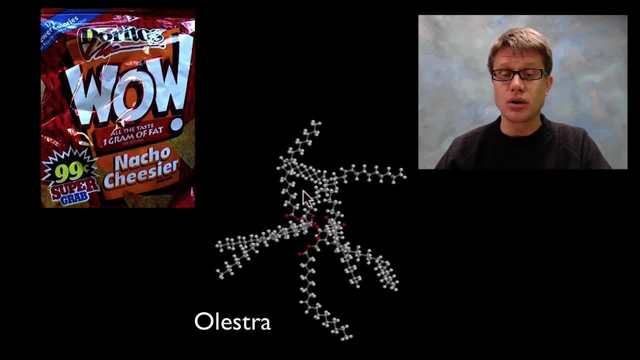 did is took a normal triglyceride but they built it around a sucrose And basically they gross. So they built it around a sugar And so instead of having just 3 of these fatty acid tails, they had sometimes 8,, sometimes 10,, sometimes even more. What's neat about? 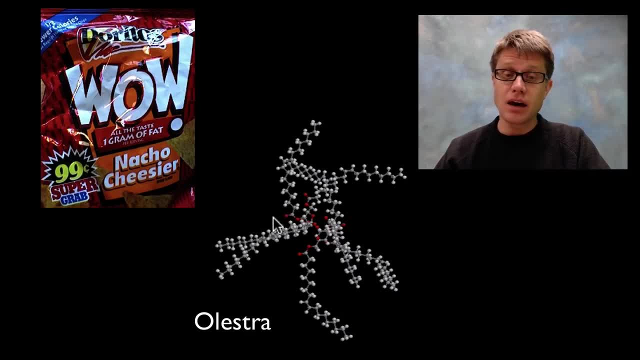 that is that when you go through your digestive system, we don't have olesterase, We don't have an enzyme that can break that down, And so the olestra moves right through our digestive system. So it's a fat that feels like a fat, tastes like a fat, but it doesn't make us 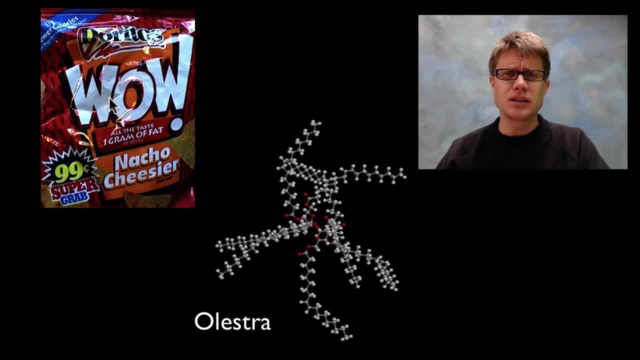 fat, And so wow chips were introduced, I think in the 1990's, and had this olestra in it today, And basically what happened is when people started eating these wow chips, they got incredibly sick, They got cramping and they had to put a warning label on the outside. 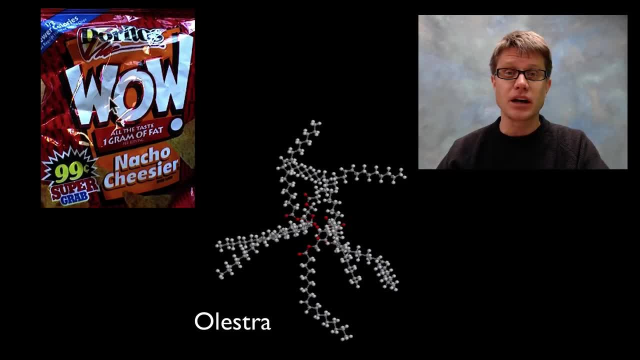 that it can lead to loose stools and it pulls vitamins outside of your body. They've kind of refined this since then, And so there's not a lot of these adverse reactions. I think Pringles like light chips still contain olestra in it, But we're tricking our body because 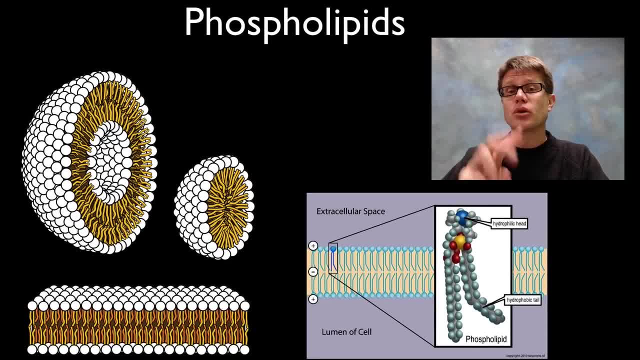